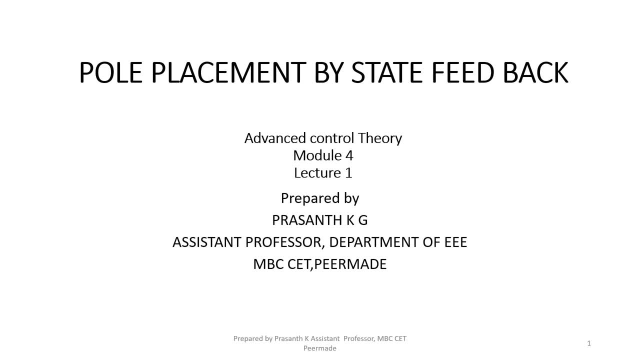 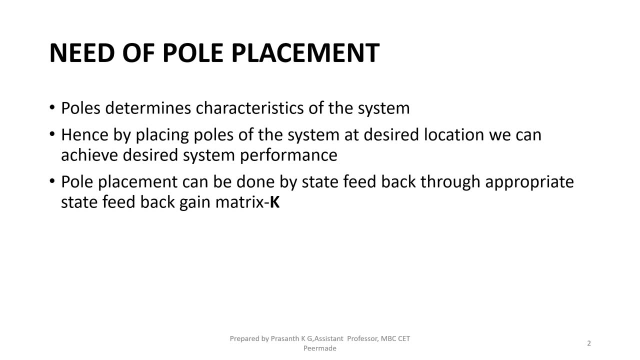 in department of Tripoli from MBC CET pyramid. So let us start. First of all, we will discuss what is the need of pole placement. So we have already discussed poles determines the characteristics of the system. We have defined the stability of the system based on location of poles. If all poles of the system 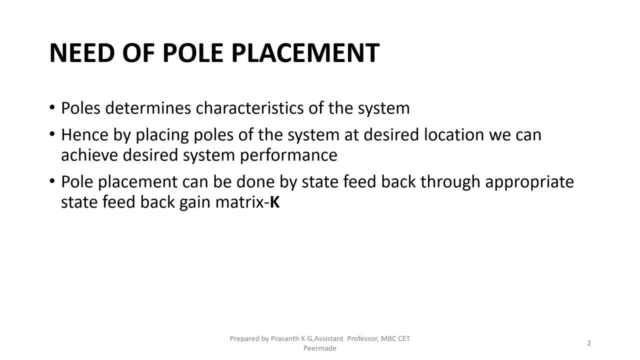 are on left side of j omega axis in S plane, then the system is stable. If at least one pole exists on the right half of S plane, then the system will be unstable. If pole pace exists on j omega axis, then it is unstable. If pole pace exists on j omega axis, then it is unstable. 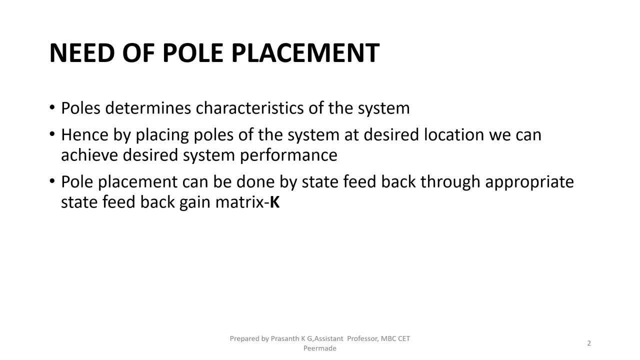 omega axis and the remaining poles are on left side of j omega axis, then the system is said to be marginally stable and the output will be oscillatory. So the stability of the system is depending upon location of poles. Also, we know all time domain specifications like rise time. 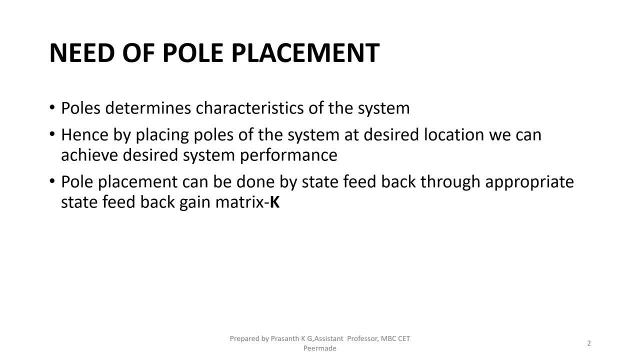 peak time, steady state, error, peak overshoot, and all these parameters are depending upon the location of poles. By placing the closed loop poles of the system at desired location, we can achieve the designed system performance. So pole placement. this pole placement can be done by: 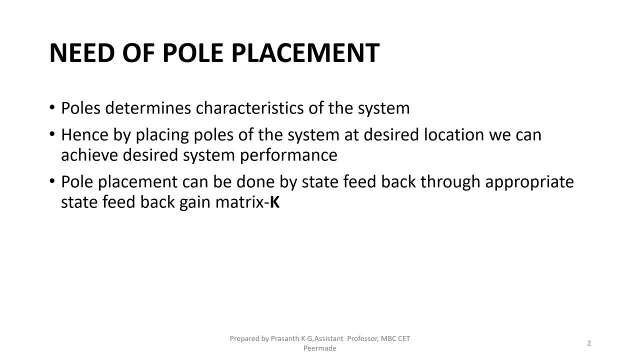 state feedback through appropriate state feedback gain matrix. So this is the requirement. So for improving the system performance, we need to design a state feedback gain matrix. In module 1, we have designed a state feedback gain matrix. In module 2, we have designed a state feedback gain matrix. 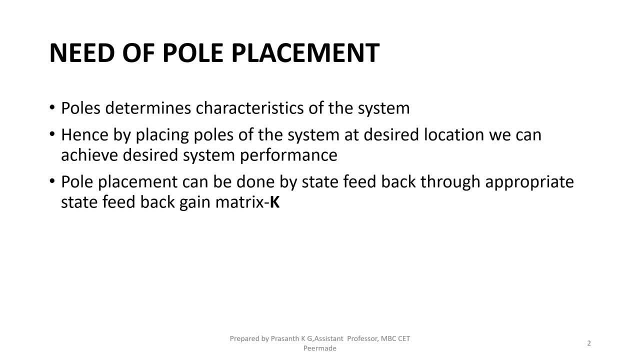 In module 3 we have discussed one more method for improving the performance of the system, that is by imposing controllers. So we have seen that by introducing proportional controller rise, time reduces. By introducing integral controller the steady state error is reduced. By introducing a derivative controller that is increasing kd, the damping is improved and oscillatory response is. 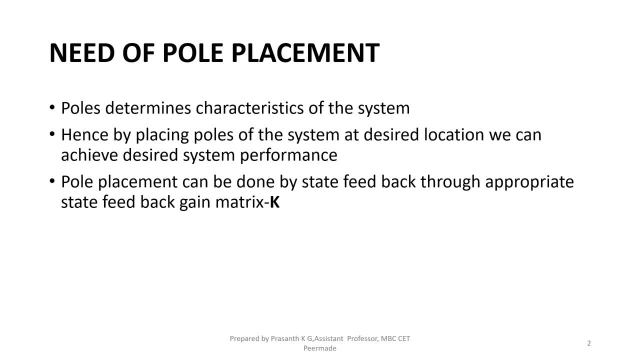 reduced, Peak overshoot is reduced. So we have seen that by introducing proportional controller, rise time is reduced. So for a higher order system, this pole placement technique is a better method than our classical method, that is, by using controllers. So that is why, for higher order, 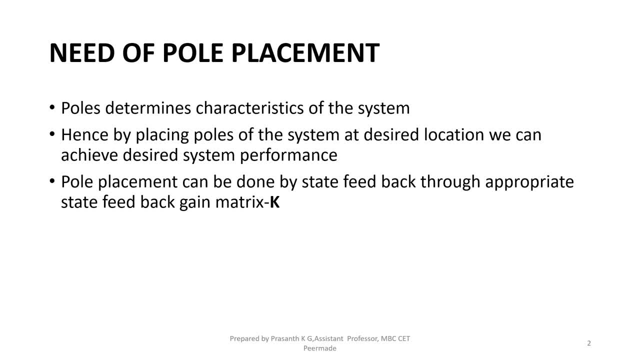 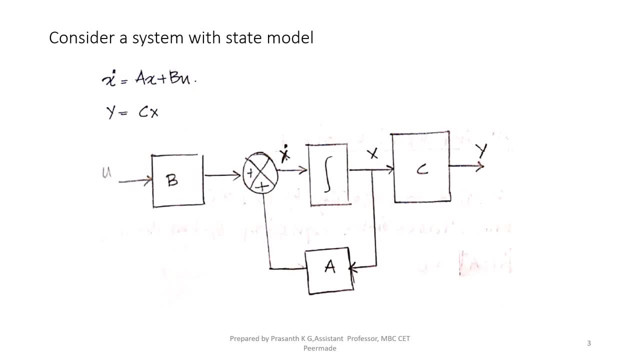 systems. we will go for pole placement than the controllers. The block diagram of this standard system. Consider a system with state equation x, dot, x dot equal to ax plus bu and y is equal to cx, Where a is the system matrix and b is the input. 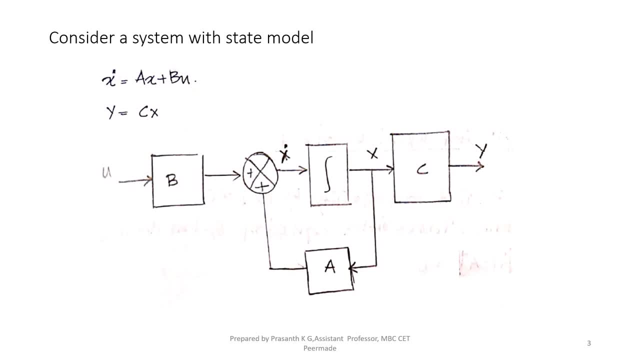 matrix c is the output, matrix x is the state vector and u is the input. As you can see, this equation, x dot equal to ax plus bu, Here you have x dot and here you have u. So b and u multiplied here you will get bu. Similarly, if you are integrating x dot, you will get x. state of the. 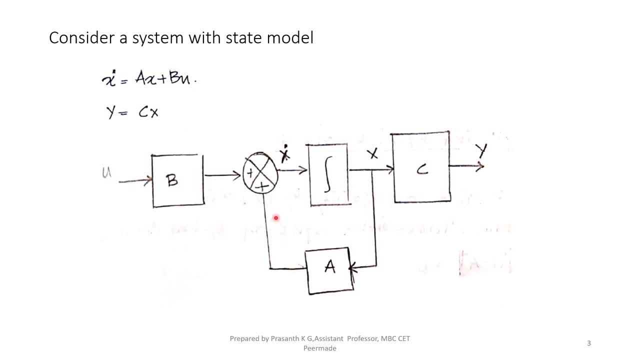 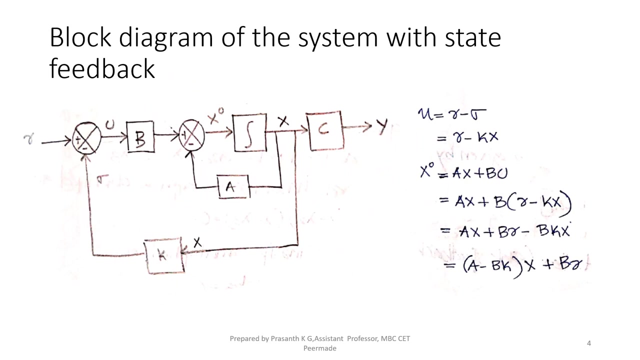 matrix and if you are feeding it back through system matrix a, you will get ax here. So x dot will be equal to ax plus bu. Similarly y equal to cx. that is here you have the state of the matrix x and here you have the c. So c into x, y is equal to cx. If I am having a control law like this u. 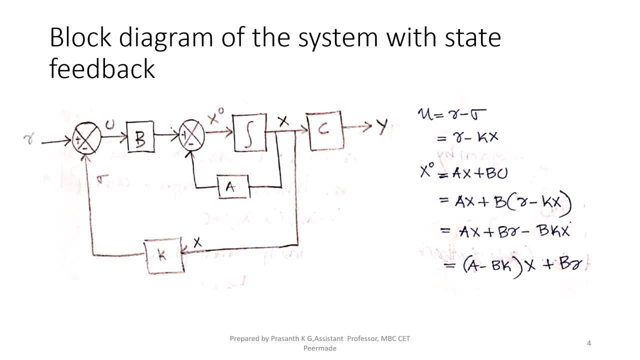 equal to r minus kx. I can impose state feedback gain matrix k here. So now the input of the system is r, k is the state feedback gain. matrix x is the state of the system. it is feedback. through this loop Now you can see that u is nothing but r minus sigma and sigma is nothing but k into x. 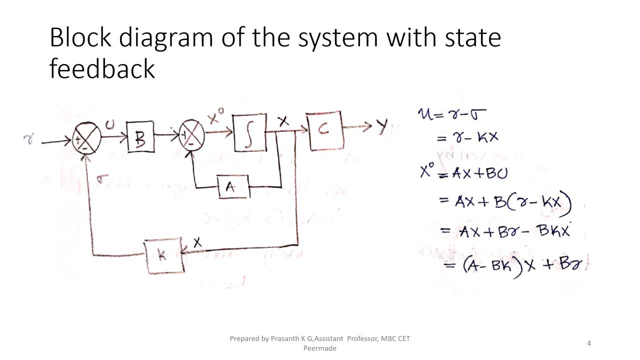 So the control law will become u equal to r minus kx. Now the state equation of the system, x dot equal to ax plus bu. But instead of u you have r minus kx here. If you are substituting that here, you will get ax plus br. If you are opening this bracket, you will get br minus bkx. You can. 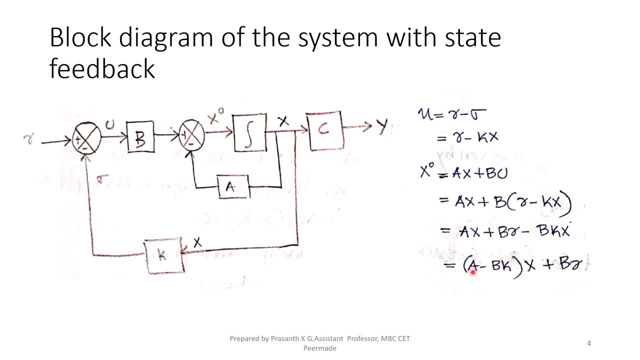 take state of the matrix x common. here and now the equation will become a minus bk into x plus br. There is no change in the output equation since y is equal to c into x, But the state equation is. that is, a system matrix is modified as a minus bk. Previously it was only ax plus bu, Now it is a. 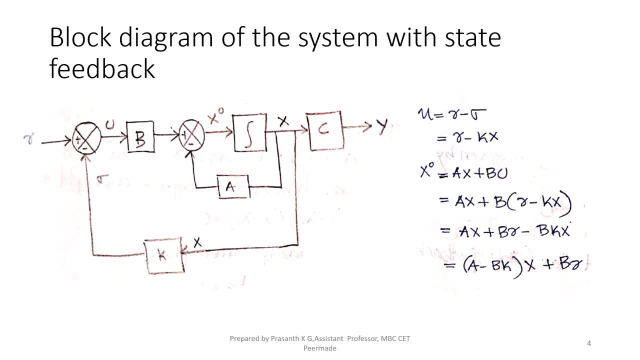 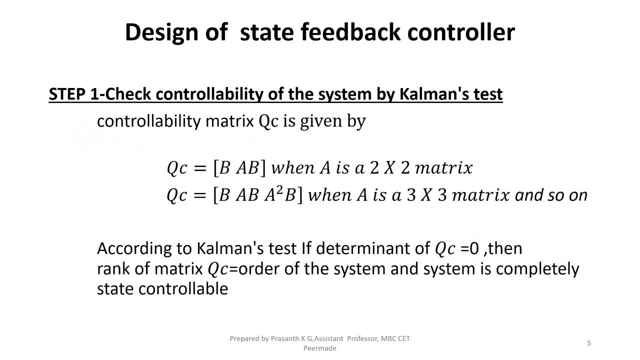 minus bk into x plus br. So this is how, with the state feedback, the state equation of the system is improved. Now we will see what are the different steps that are involved in the design of state feedback controller. So the necessary and sufficient condition for design of state feedback controller is: 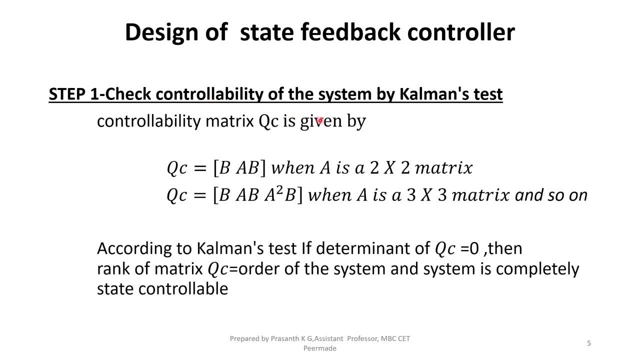 checking the controllability of the system. If the system is completely state controller, then only we can design state feedback controller. So the first step will be checking the controllability of the system which we can use, which we can do by Kalman's test. As we have already said, we have 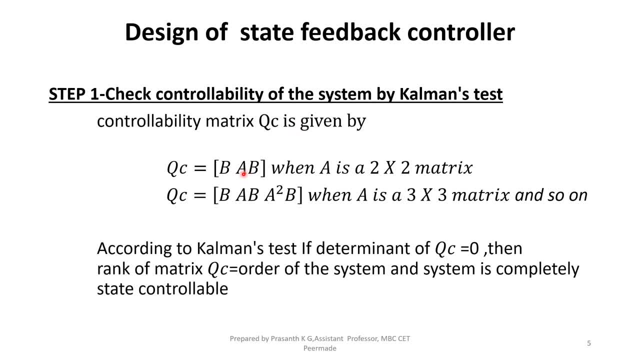 defined the controllability matrix qc as qc equal to b, ab, a square b, etc. For a 2 by 2 system matrix, we have two terms only: b and ab. For a 3 by 3 system, we have qc equal to b, ab and a square b. 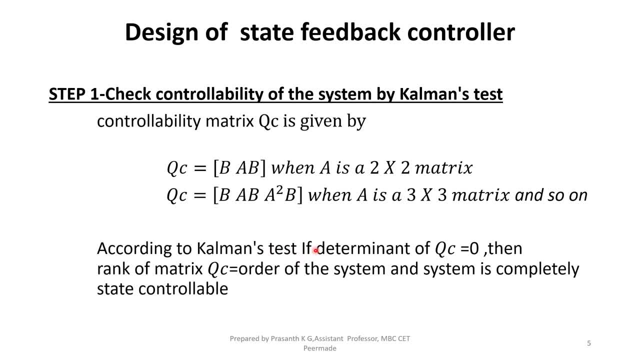 Three terms will be there Now. according to Kalman's test, if the determinant of the qc equal to 0, then rank of the matrix qc will be equal to order of the system, and system is said to be completely state controlled. So this is what the first step involved in the design of state feedback. 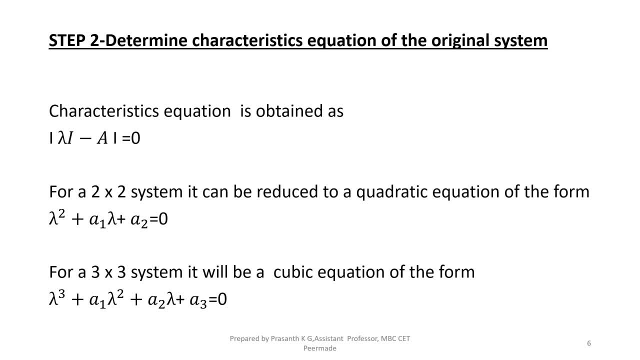 controller Determining the characteristic equation of the original system. We have already seen in your max class that characteristic equation of a system is obtained by determinant of lambda i minus a equal to 0. For a 2 by 2 system, if you are solving this equation, you will obtain a quadratic equation. 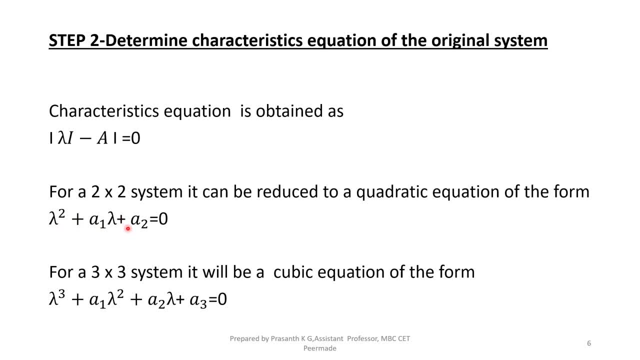 like this: lambda square plus a1, lambda plus a2, equal to 0, where a1 and a2 are constants. that is, coefficients of lambda, coefficient of lambda and the constant term For a 3 by 3 system. if you are solving determinant of lambda i minus a equal to 0, you will get a. 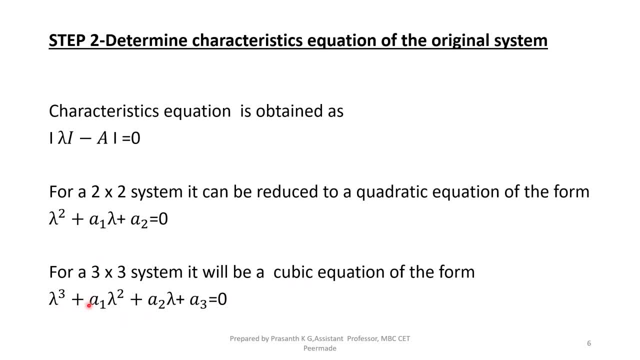 cubic equation in the form lambda q plus a1, lambda square plus a2, lambda plus a3, equal to 0.. So remember, these are the coefficients: a1- a2 in case of 2 by 2 system a1- a2 and a3 in case of a. 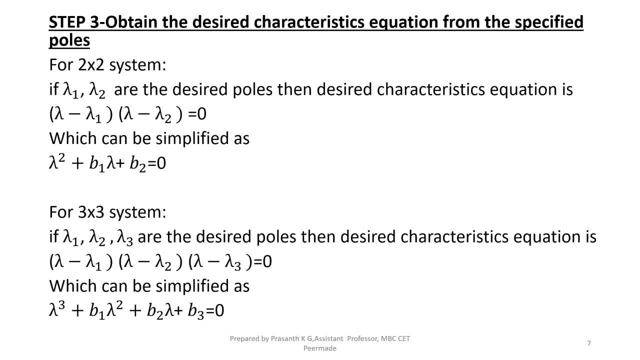 3 by 3 system. Now we will see what is the third step. Step 3 is to obtain the desired characteristic equation from the specified poles. So usually in the design criteria they will specify what are the desired location, what are the desired pole locations. So for a 2 by 2 system you will be 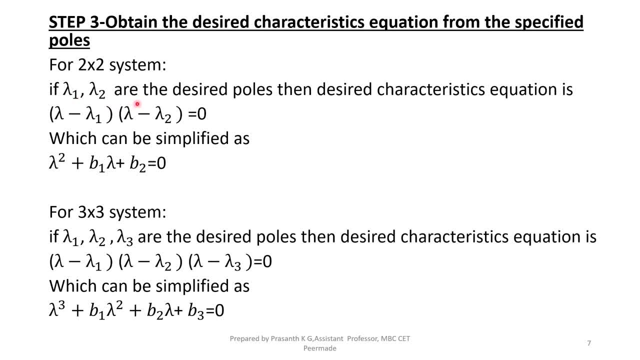 having two poles. let it be lambda 1 and lambda 2.. So if lambda 1, lambda 2 are the desired poles, you can obtain the characteristic equation of the desired system as lambda minus lambda 1 into lambda minus lambda 2, equal to 0. So if you are simplifying this equation, you will get a quadratic. 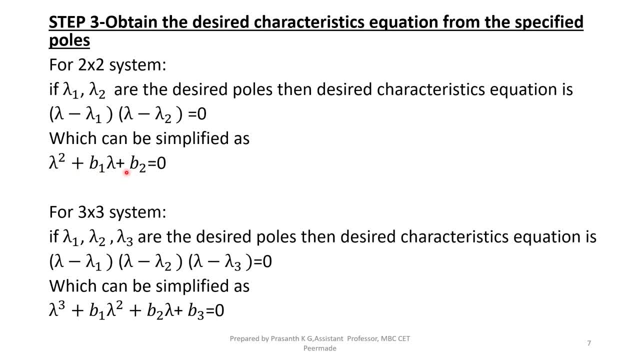 equation like square plus b1, lambda plus b2, equal to 0.. Similarly for a 3 by 3 system, that is, if system matrix is of order 3, there will be 3 desired poles. Let the poles be lambda 1,. 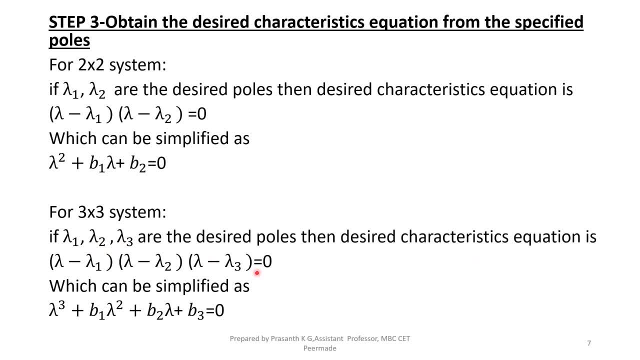 lambda 2 and lambda 3.. Then the desired characteristic equation will be obtained as lambda minus lambda 1 into lambda minus lambda 2, into lambda minus lambda 3, equal to 0, which can be further simplified as a cubic equation in the form: lambda cube plus b1. lambda square plus b2. 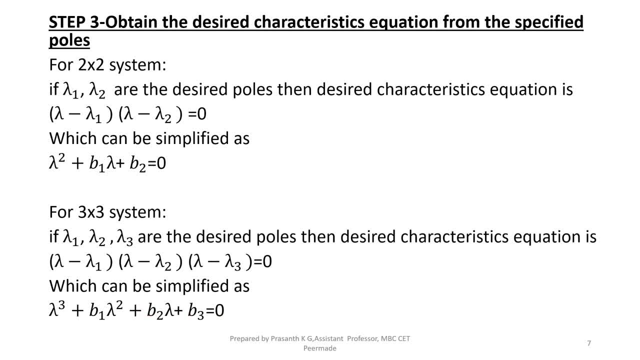 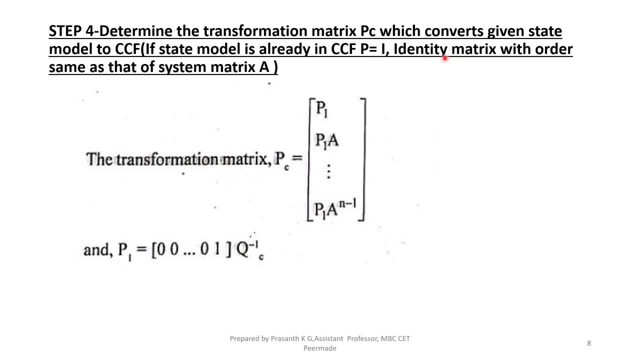 lambda plus b3 equal to 0.. The fourth step is to determine the transformation matrix, PC, which converts the given state model into controllable canonical form. It is important that you have to see how you can identify whether the state model is in controllable. 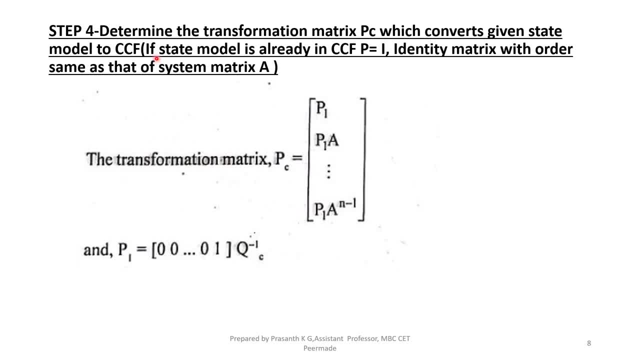 canonical form that we will discuss while we are doing the problems. So if the state model is already in controllable canonical form, PC matrix will be equal to I, that is, identity matrix, with the order same as the order of the system, matrix A. So in generally, 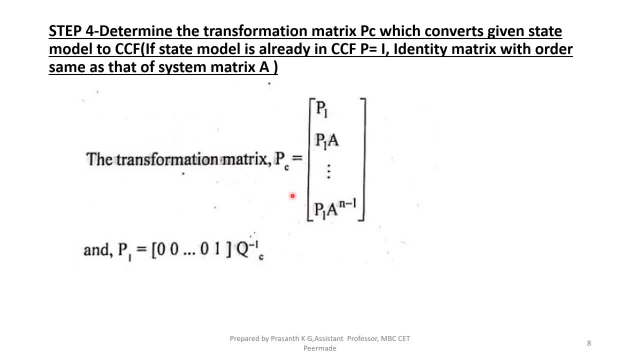 the transformation matrix PC is given as a row matrix P1, P1A. P1A square like that P1 into A raised to n minus 1, where P1 equal to 0,, 0,, 0 and last element will be 1. 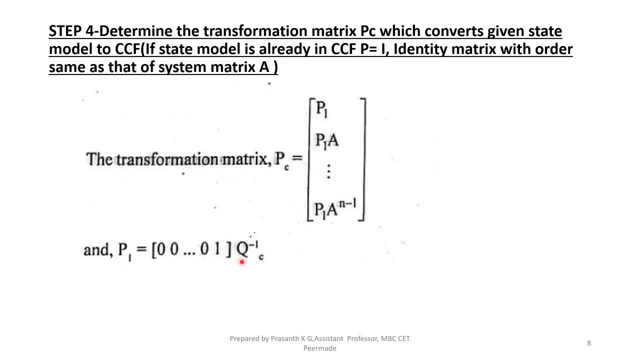 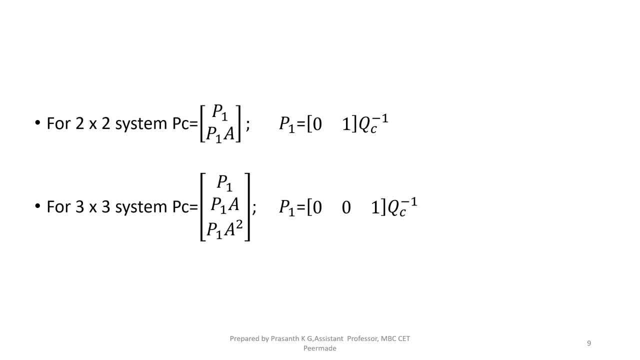 into Q1. So Q1 is equal to QC inverse. This QC is nothing but the controllability matrix that you have already obtained in step 1.. For a 2 by 2 systems, PC will have only two terms. First element will be P1 and the second row element will be P1 into A and P1 will be. 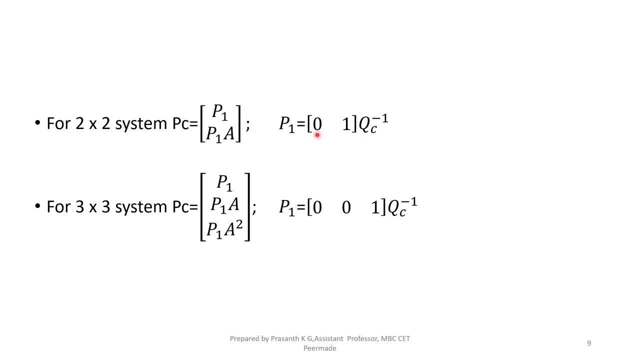 equal to 01 into QC inverse. You can see that there is only two elements in this row matrix. For a 3 by 3 system, PC will have only two terms. So QC will have only two terms. For a 3 by 3 system, PC will have only two elements. 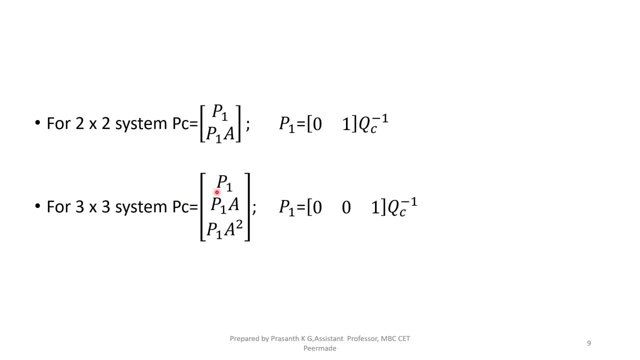 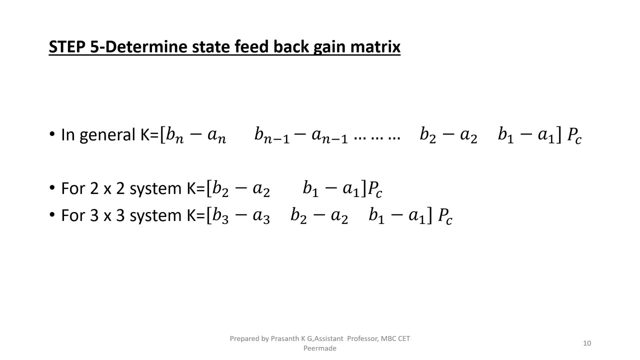 Pc will have three elements, that is, three rows. First row will be P1,. second row will be P1a. third row will be P1 into a square where P1 equal to 001 into Qc. You have to remember these equations Now. the last step is obtaining the state feedback gain matrix. So this is the general 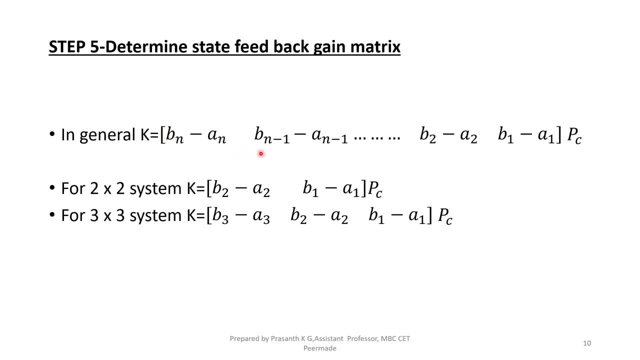 equation K is equal to: first element is Bn minus An. second element is Bn minus 1 minus An minus 1, etc. up to B2 minus A2 and last element will be B1 minus A1. into Pc matrix For a two by two system. 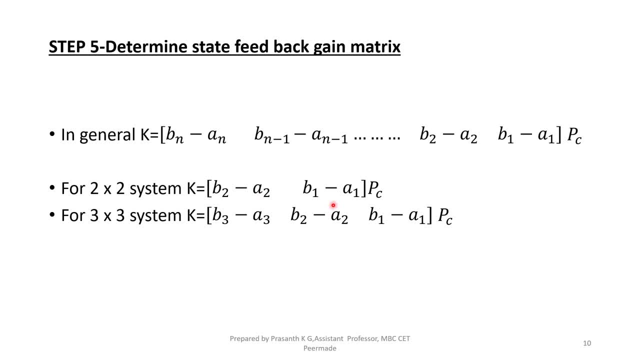 you will have two elements. First element will be B2 minus A2, second element will be B1 minus A1 into Pc. So for a three by three system, your state feedback gain. matrix is given, as K is equal to B3 minus A3,. second element, B2 minus A1 into Pc. So for a three by three system, your state feedback gain. 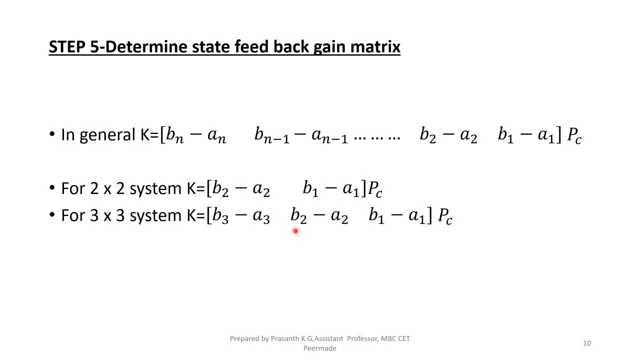 matrix is given as: K is equal to B1 minus A2 and the third element is B1 minus A1. Here, B1, B2 and B3 are coefficients of desired characteristics polynomial, and A3, A2, A1 are coefficients of. 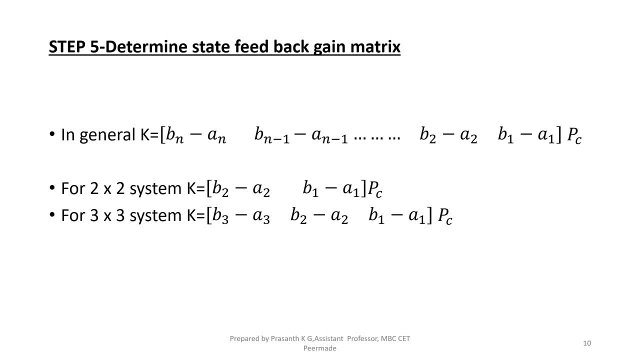 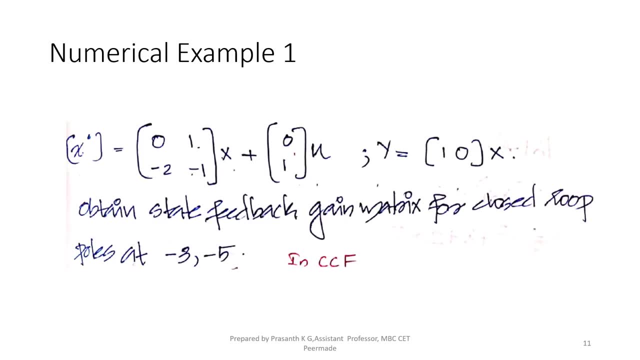 the characteristics equation of the present system. So these are the five steps which are involved in the design of state feedback gain. Now we will see some numerical examples based on that. So this is the state equation of the system given X dot equal to system matrix 0, 1 minus 2 minus 1 into X, plus 0, 1 into U and Y is equal to: 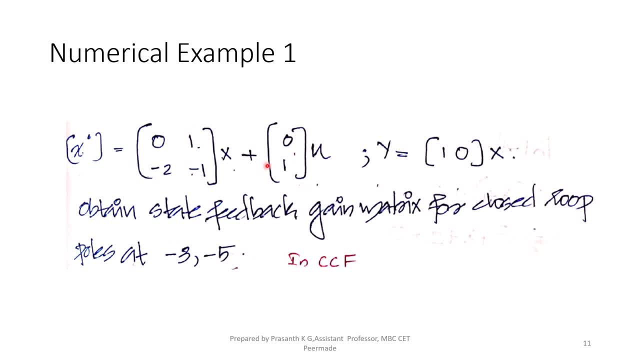 row matrix 1, 0 into X. So this is the state equation and this is the output equation. Now the question is to obtain the state feedback gain matrix for closed group poles as minus 3 and minus 5.. So these are the two desired fold operations. Now, by seeing the question itself, 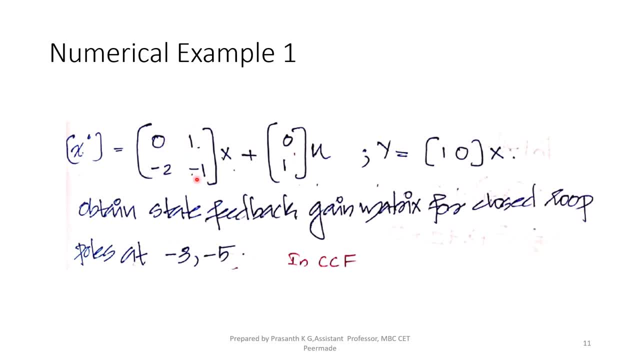 you can see: the first row is 0, 1 and the second row is 0, 1 and the third row is 0, 1 and the second row is minus 2, minus 1 and the B matrix is like: all the elements are 0s except the last. 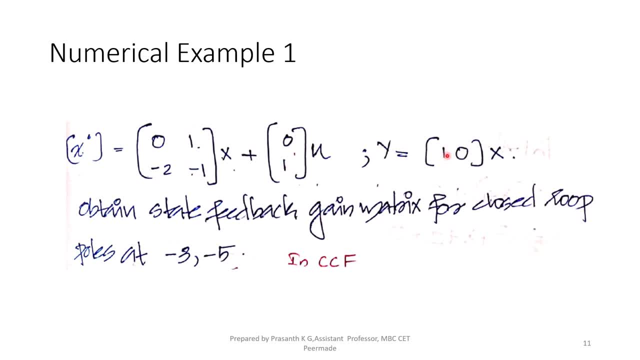 row which is having 1.. Now Y is equal to first element is 1 and all remaining, all elements are 0.. This is the property of condolable canonical form. So the system state model which is given is already in condolable canonical form. This by which we this we will require in your step. 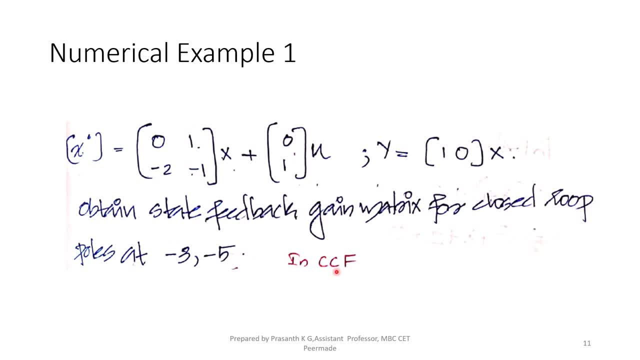 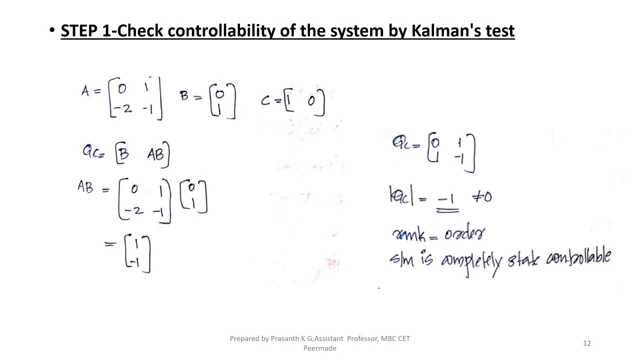 where we calculate PC. There is no need to calculate PC here because the state model is already in condolable canonical. Now we will see step 1, that is, taking the condolability of the system. by Kalman's test You have the state system. matrix A is equal to 0, 1 minus 2 minus 3. 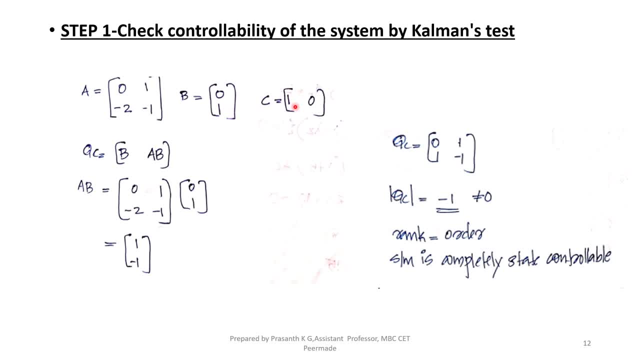 input matrix B is equal to 0, 1 and C equal to minus 0.. Now for a 2 by 2 system. we have condolability matrix QC equal to B and AB. B is nothing but 0, 1.. So you have to calculate the. 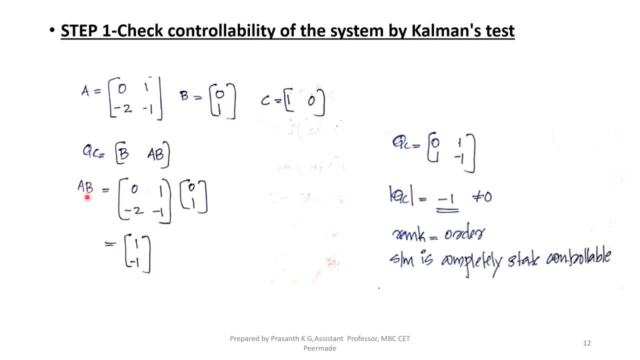 second row matrix, B is equal to 0, 1 and C equal to minus 0.. Now for a 2 by 2 system. we have second row, second column, like AB, A is given, B is given here. So if you are substituting and. 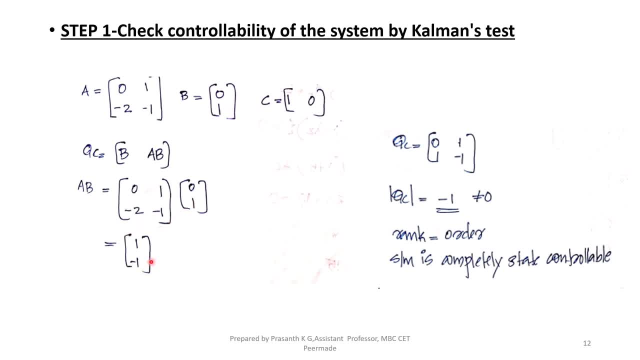 multiplying these two, you will get the AB. Now, if you are substituting B as well as AB, you will get the QC matrix. like this: If you are taking the determinant of this QC matrix- determinant of QC equal to 0, into minus 1, minus 1 into 1, that is equal to minus 1.. You can see that QC determinant. 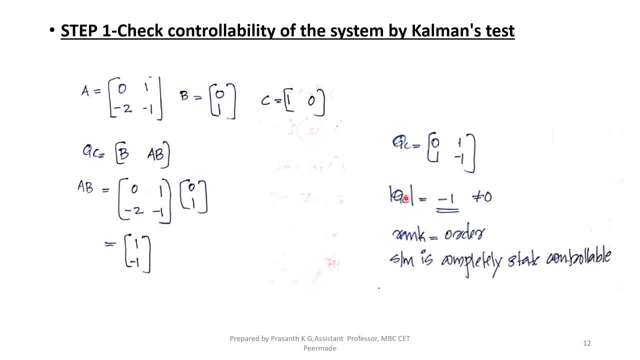 of QC equal to 0, which means the rank of matrix QC equal to order of the system equal to 2.. So system is completely state controllable according to Kalman's test. Now the necessary and sufficient condition for designing, for place designing the state feedback gain matrix, is achieved. 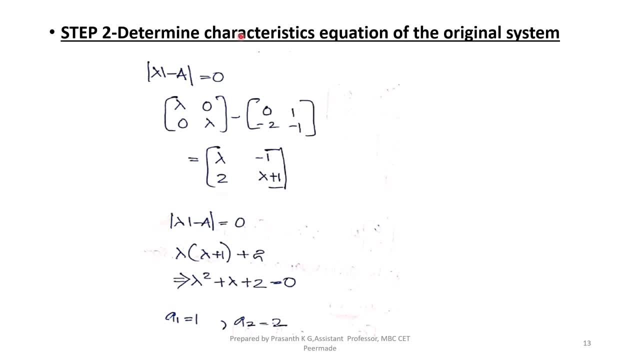 Determining the characteristic equation of the original system, So determinant of lambda. I minus A, equal to 0.. If you are substituting lambda into 1, 0, 0, 1, since your system is of 2, order 2, I is also of order 2. 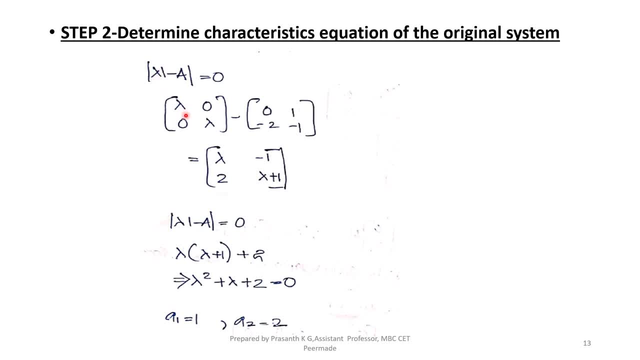 that is 1, 0 into 0, 1. If you are multiplying lambda I, it will be lambda 0, 0 minus 0, sorry, lambda minus. Now the system matrix is given as 0, 1 minus 2 and minus 2.. If you are simplifying that, 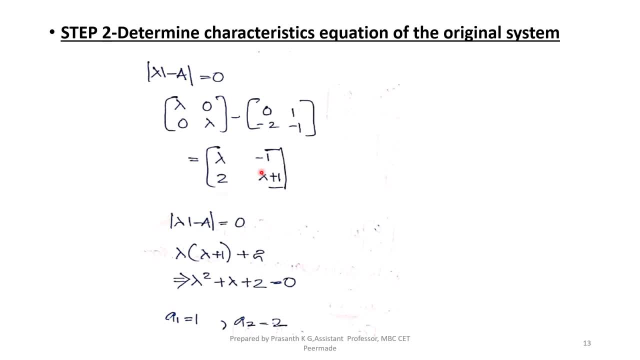 you will get lambda I minus A equal to lambda minus 1, 2 and lambda minus 1 minus 2.. So if you are equating determinant of lambda I minus A equal to 0, you will get an equation like this: that is, lambda into lambda plus 1 minus 2 into minus 1, which is equal to lambda square plus lambda plus. 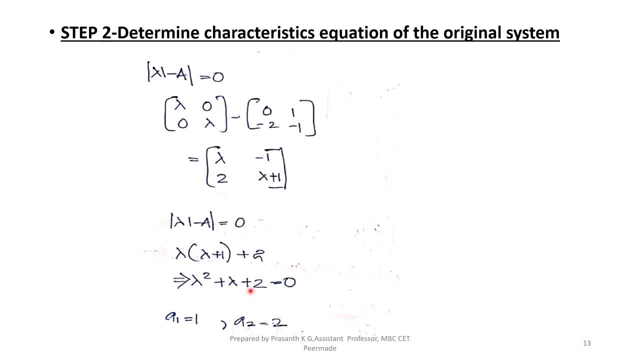 2 equal to 0.. So you can see the coefficients of this system, this polynomial as. So. here the coefficient is 1, that is A1 equal to 1.. Here the coefficient is a constant term, is 2.. So A2 equal to. 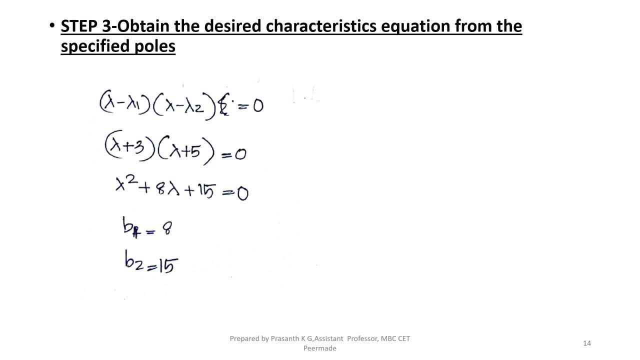 1.. Now for step 3, obtaining the desired characteristic equation from the specified poles. So the specified poles are given in your question as minus 3 and minus 5.. So lambda 1 is equal to minus 3 and lambda 2 equal to minus 5. Lambda minus lambda 1 is lambda minus lambda 2. 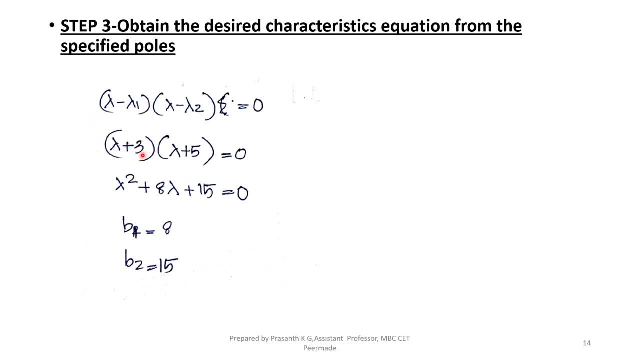 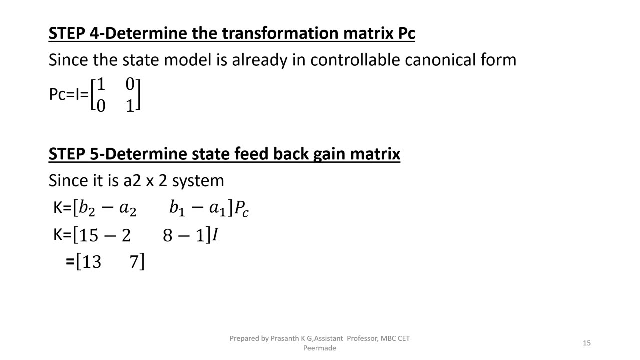 equal to 0. If you are substituting lambda 1 and lambda 2, you will get a quadratic equation like this: So now you can see the coefficient and constant terms are P1 equal to 8 and B2 equal to 50.. We can proceed to step 4, that is, determining the transformation. 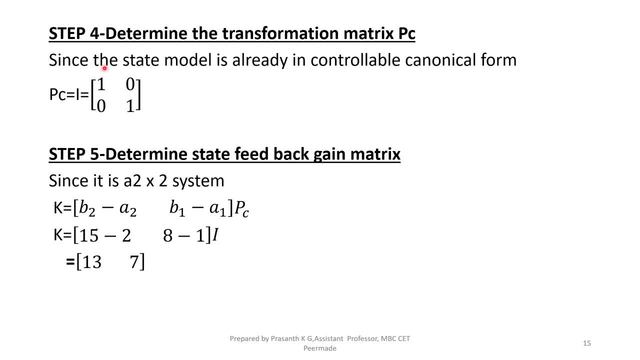 matrix. I have already shown that the state motor is in controllable canonical form. There is no need to find the PC matrix. PC matrix will be the identity matrix of order 2 by 2, that is 1, 0 into 0, 1.. So we can proceed to step 5, that is, determining the state feedback gain matrix. 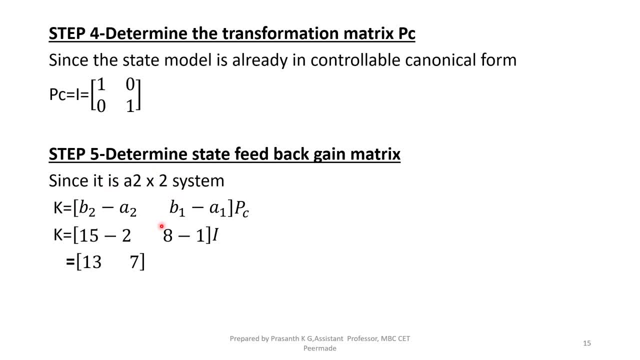 So, since it is a 2 by 2 system, you have only two elements, that is, B2 minus A2 and B1 minus A1, into PC. So B2, you have 15, A2 you have 2, B1 equal to 8 and A1 equal to 1.. If you are, 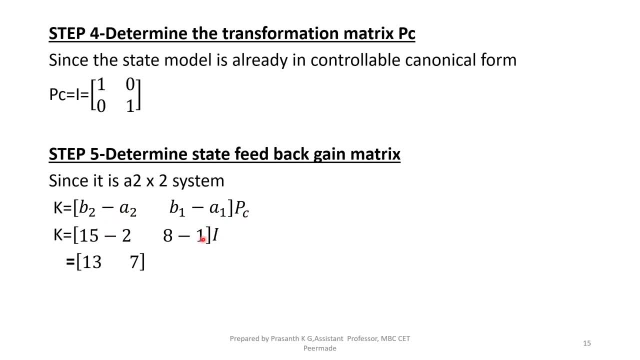 substituting all values in PC. since PC equal to I no need to multiply this. any matrix into identity matrix will be the same matrix, So it will be 13 and 8,, 13 and 7.. So these are the two elements in your state feedback gain matrix. So this is how we can design a state feedback. 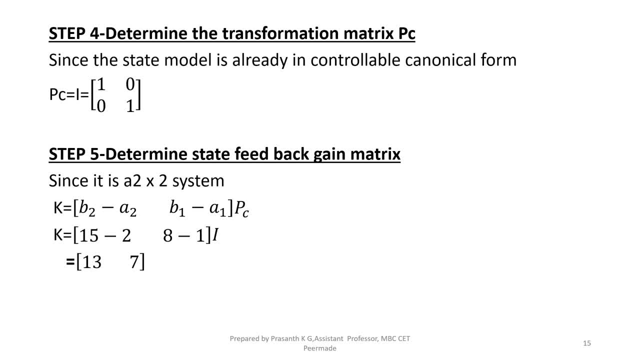 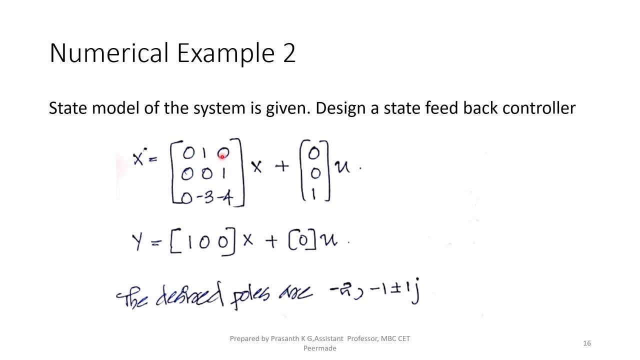 gain matrix by using for pole placement Controllable canonical form. You see the matrix 0, 1, 0, 0, 0, 1 and the third row are some other elements. So here in input matrix the last row element should be 1, remaining element should be: 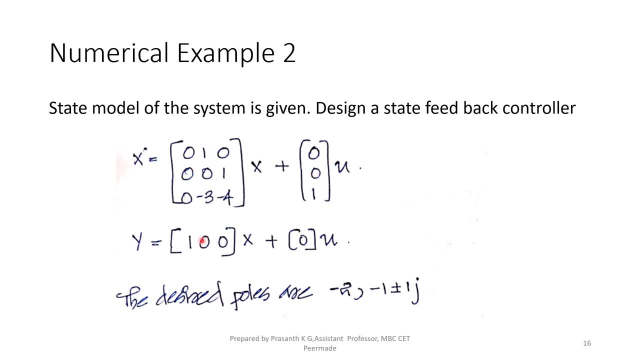 0. This is the indication of controllable canonical form. So this is the indication of controllable canonical form. Also, in C matrix, first element should be 1 and the remaining element should be 0. So this is the indication that system is in controllable canonical form. 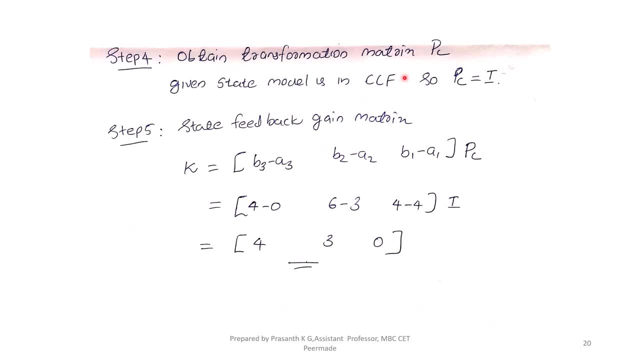 Since the system is already in controllable canonical form, PC will be I of order 3 by 3.. So step 5, state feedback gain matrix K is equal to B3 minus A3, B2 minus A2, B1 minus A1,. 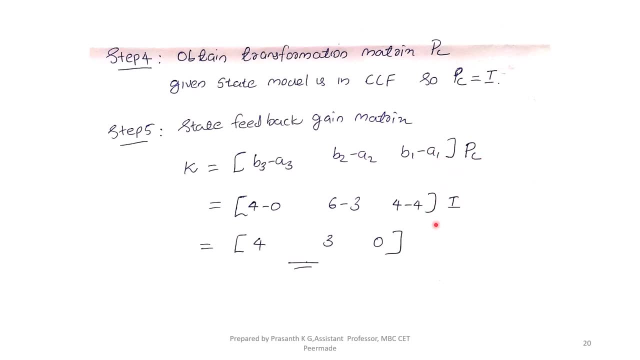 into PC. So since PC is identity matrix, no need to multiply again. it will be B3 minus A3, B2 minus A2 and B1 minus A1. So substituting the values of B3, A3, B2, A2 and B1 and A1, you will. 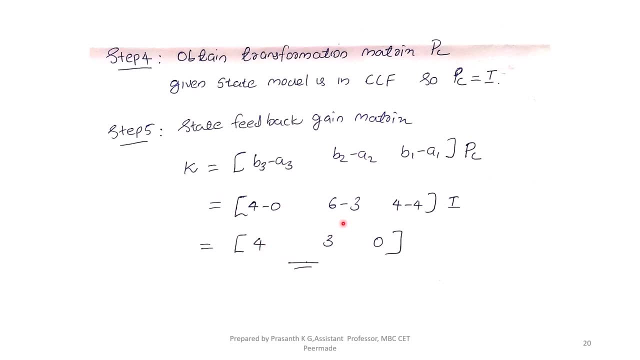 get the state feedback gain matrix as 4 minus 0,, 6 minus 3,, 4 minus 4, that is, 4, 3 and 0.. So this is the state feedback gain matrix. So this is the numerical example 2.. 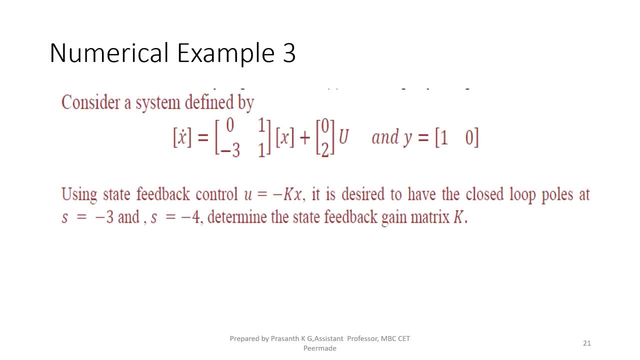 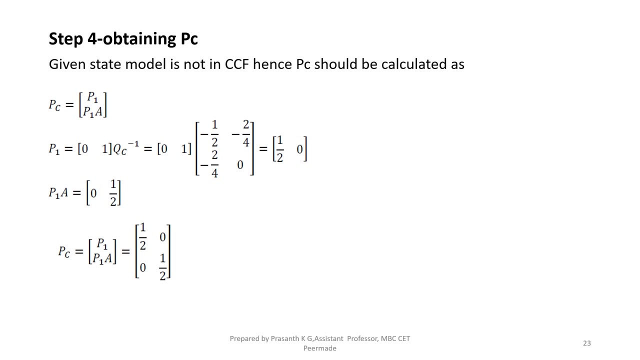 Hope it is clear. Now we will move on. Your state model is not in controllable canonical form. Whenever your state model is not in controllable canonical form, you have to calculate in step 4.. That is the difference. So we will do one more question based on this. 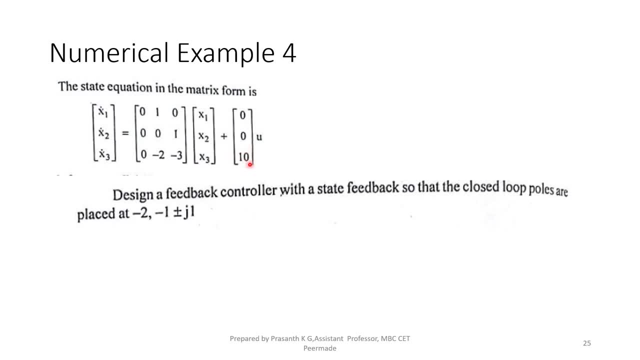 If this element was 1, the system will be in controllable canonical form. So you have a scaling of 10 here. So if this element was 1, the system will be in controllable canonical form. that is the case you have to take. if it was 1, PC will be equal to identity matrix, isn't it? 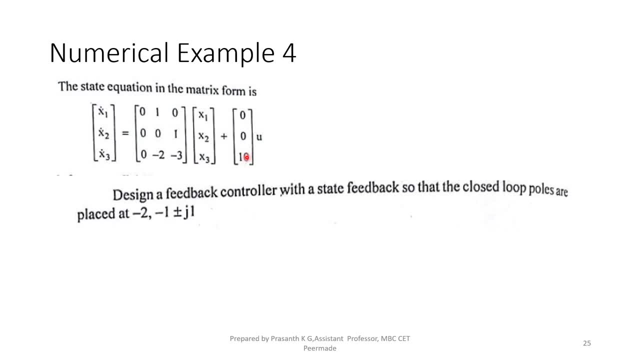 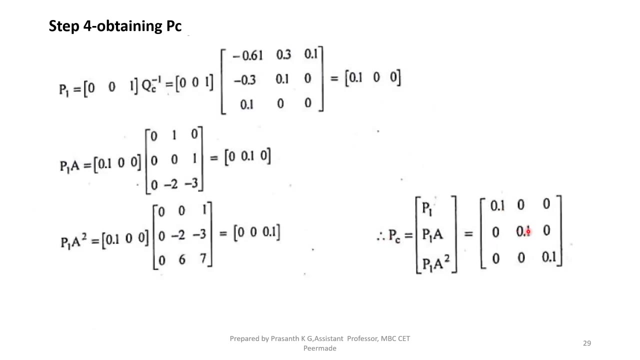 1, 0, 0, 0, 1, 0 and 0, 0, 1.. So since you have 10 instead of 1, you have to divide the entire PC matrix with 10.. Now you write 10.. So this is what PC equal to 0.1, 0.1, 0.1,.